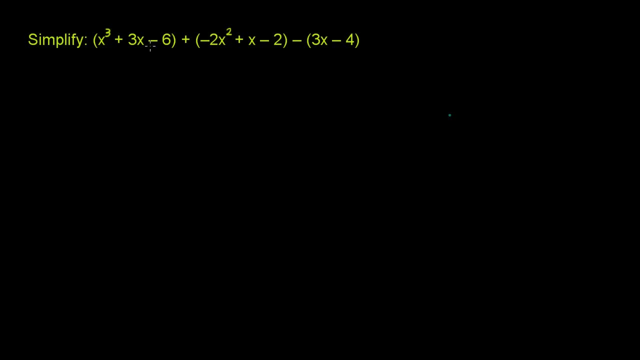 So a good place to start. we'll just rewrite this and see if we can eliminate the parentheses in this step. So we'll first just start at the beginning. We have the x to the third right over there, So x to the third and then plus 3x. 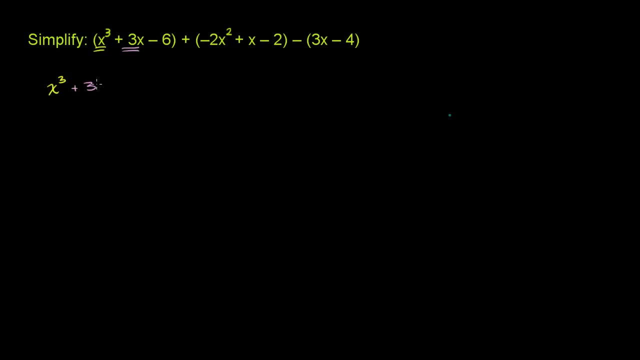 I'll do that in pink Plus 3x, And then we have a minus 6.. Now we don't have to put the parentheses around there. Those don't really change anything Plus, and we don't have to even do anything with these. 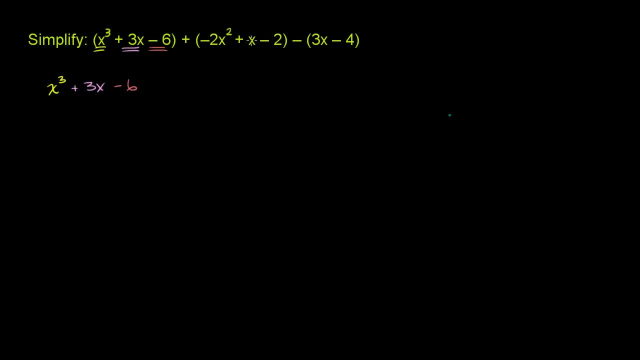 parentheses. We can eliminate them. just because there's a positive sign out here, We don't have to distribute anything. Distributing a positive sign doesn't do anything to these numbers. So then, plus, we have a negative 2x squared. So this term right here is negative 2x squared or minus. 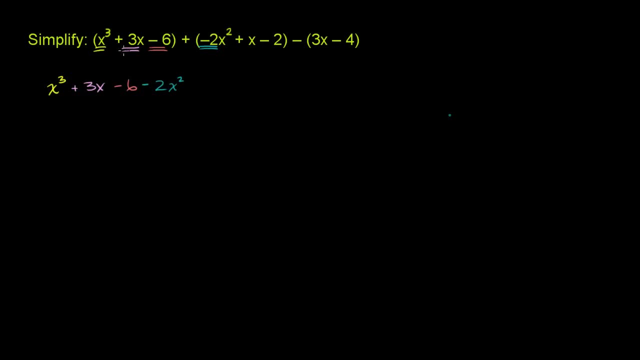 x squared, And then we have a plus, We have a plus x, We have a plus x, Then we have a minus 2.. And we have a minus 2. Then we have a negative sign times this whole expression. So we're going to have to distribute the negative sign. 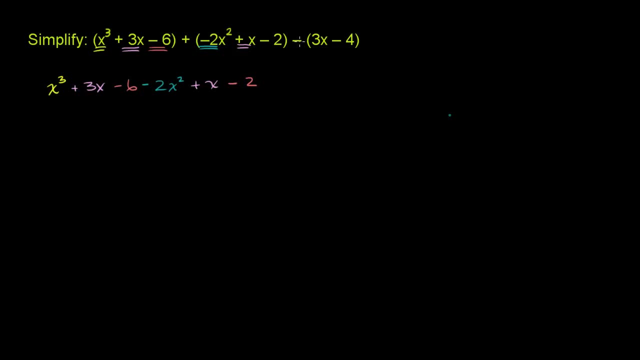 So it's a positive 3x, but it's being multiplied by negative 1.. So it's really a negative 3x. So minus 3x, Then you have a negative. you can imagine this as a negative 1 implicitly out here. 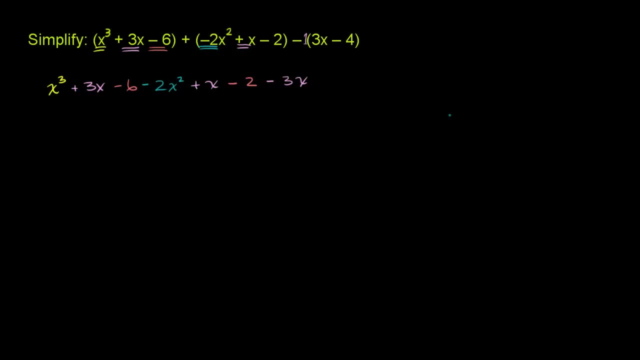 Negative 1 times negative, 4. That's a positive. 3x, That's a positive 4. So plus 4.. Now we can combine terms of similar degree, of the same degree. Now, first we have an x to the third term. 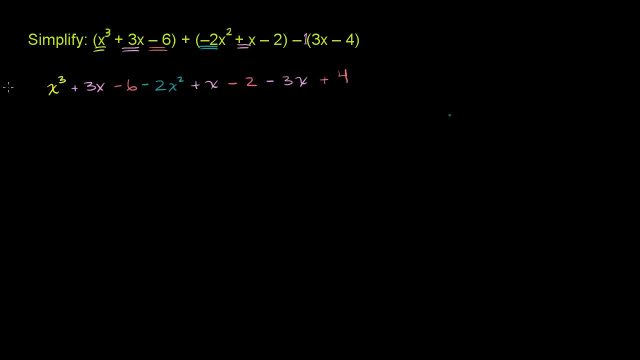 I think it's the only third degree term here, because we have x being raised to the third power. So let me just rewrite it here. We have x to the third And let's look at our x squared terms Looks like we only have 1.. 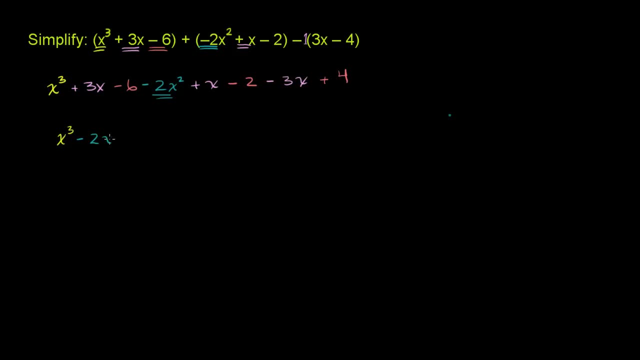 We only have this term right here. So we have minus 2x squared. And then what about our x terms? We have a 3x plus an x Minus a 3x again, So that 3x minus a 3x will cancel out and you're just.